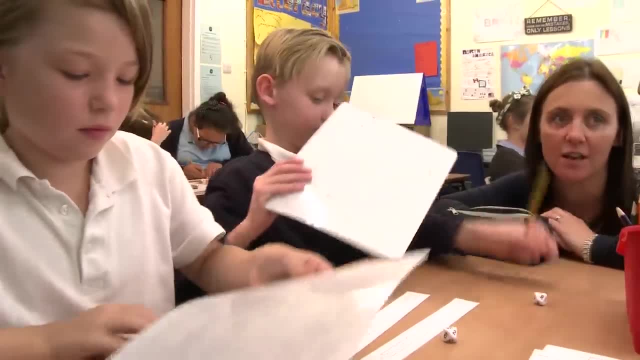 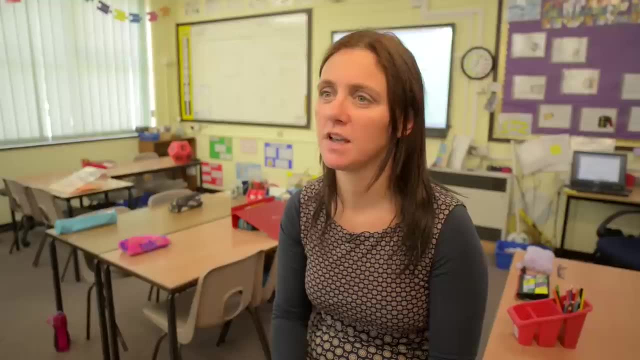 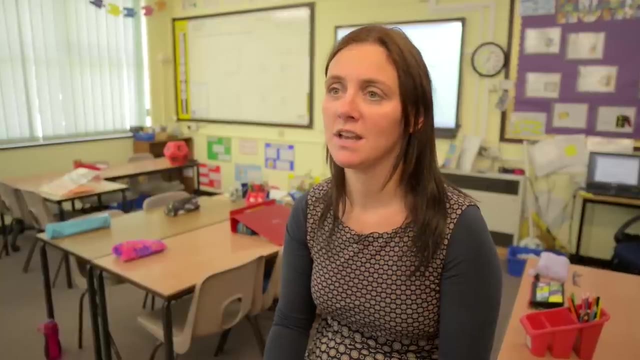 And so in Cambridge Primary Maths, problem solving is embedded throughout those four areas. Problem solving is really important in maths in terms of encouraging children to start to explain, to generalise, To reason, To justify. All of those higher order thinking skills which obviously go across the curriculum can be really enhanced in maths learning. 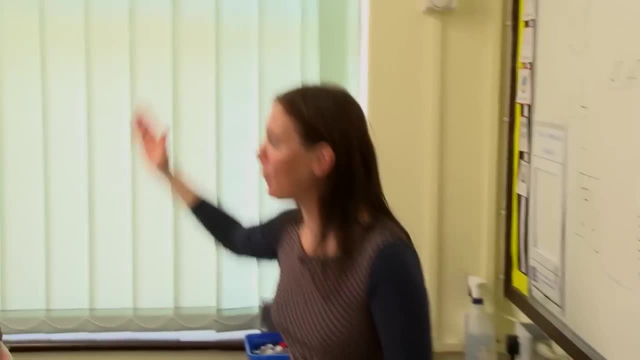 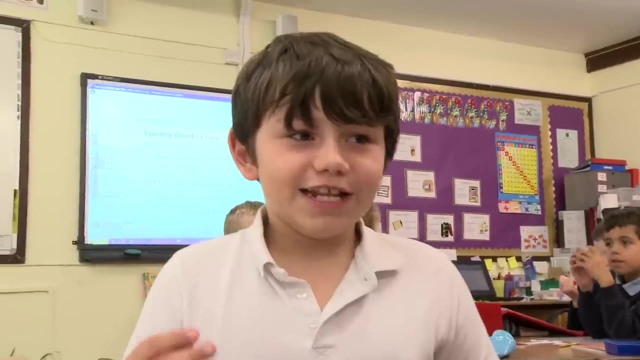 We do a lot of teaching from a kind of problem-solving angle And it does really benefit the children because it's the thinking about thinking Something was like really hard and then when you did it it was like, yes, I did it. 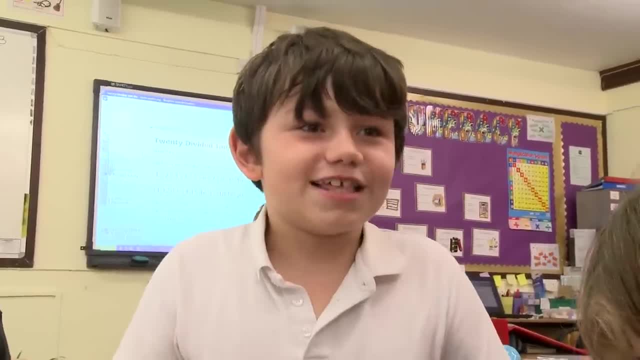 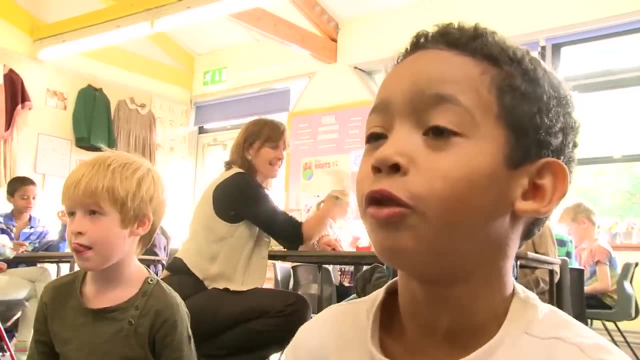 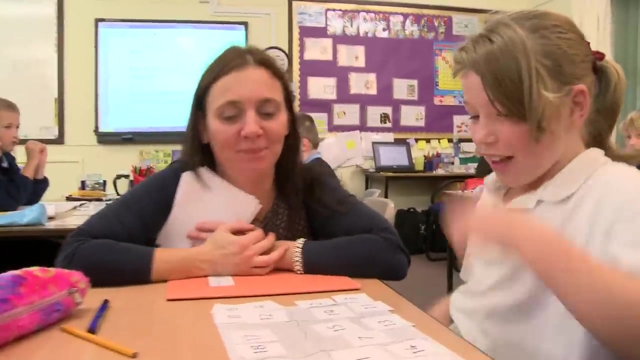 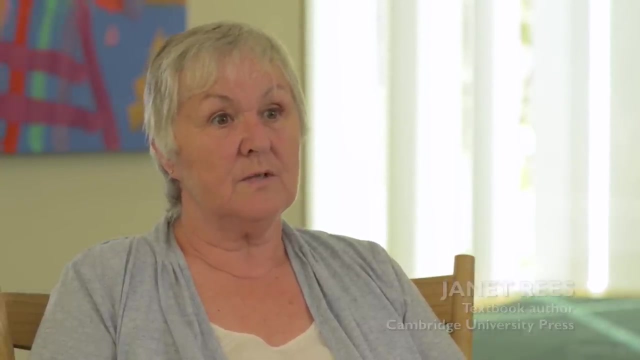 And then it was challenging, which makes it really challenging. It's fun and two hours and you can do all sorts of things with numbers. The books are written specifically for the primary Cambridge curriculum, so we work closely with that. The aim of the series is to support teachers, to help learners become confident and competent. 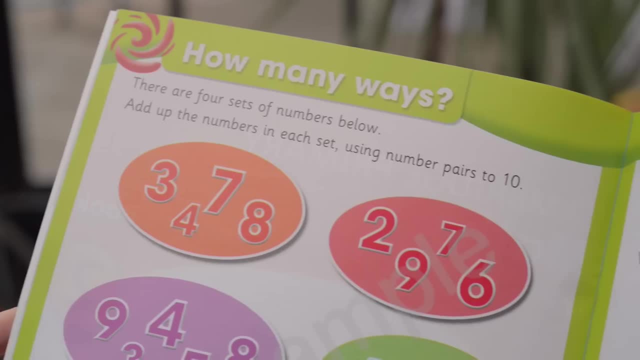 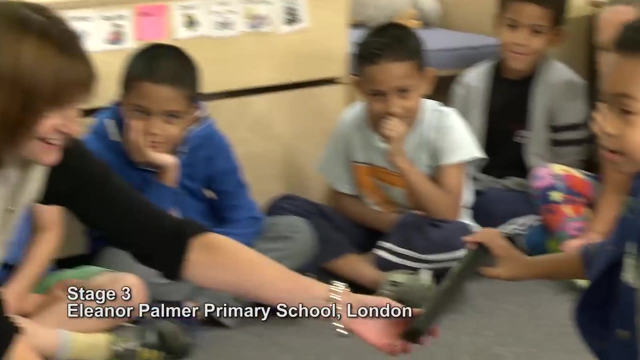 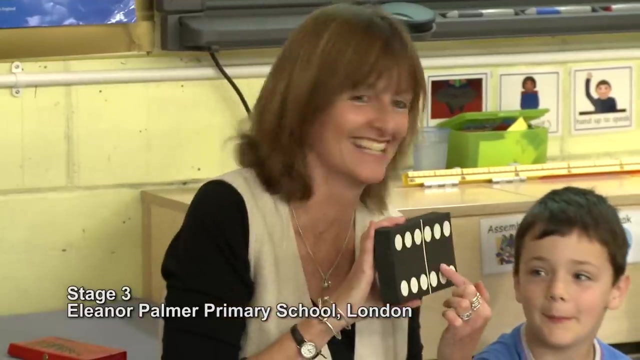 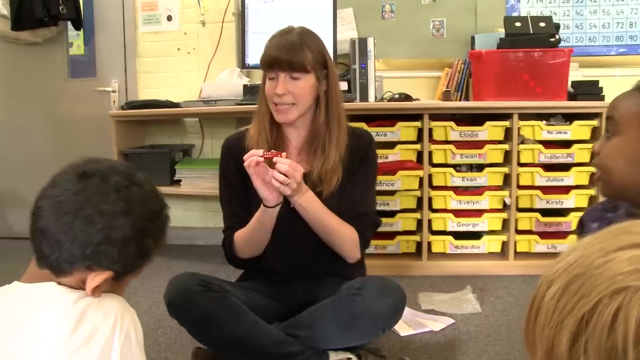 mathematicians. When we were thinking about the design of the books, we decided as a team to have games that all students, at whatever level, could play to help reinforce the mathematics. The Cambridge curriculum is dedicated to helping schools develop learners who are confident, responsible, reflective, innovative and engaged. 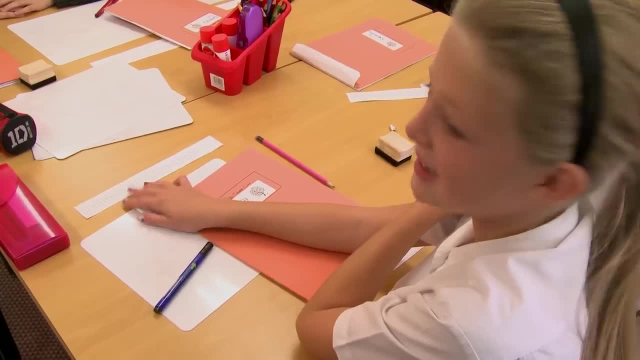 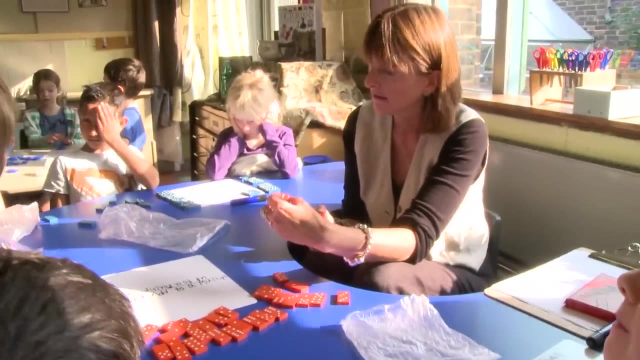 Cambridge Primary Maths is designed to nurture these attributes in learners. The domino multiplication task was from the CUP scheme and that's a really nice activity because it's doing a lot of work. It's doing what we wanted it to do, which is turn rote practice into a game. 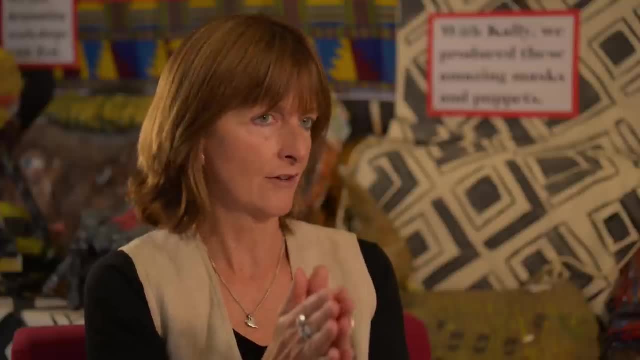 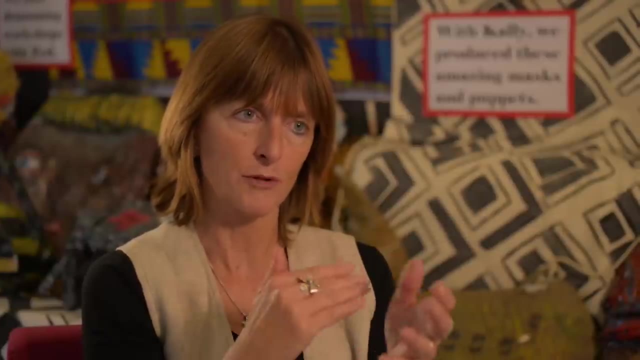 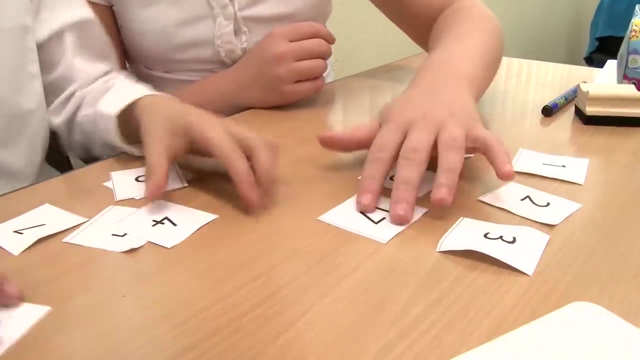 There was much more motivation. But we're very, very, very keen on the enriched materials in this school too, because they're always rich tasks, There's always lots of possibilities, There's always lots of directions you can go. Cambridge Primary Maths gives an opportunity to explore a curriculum that is international. 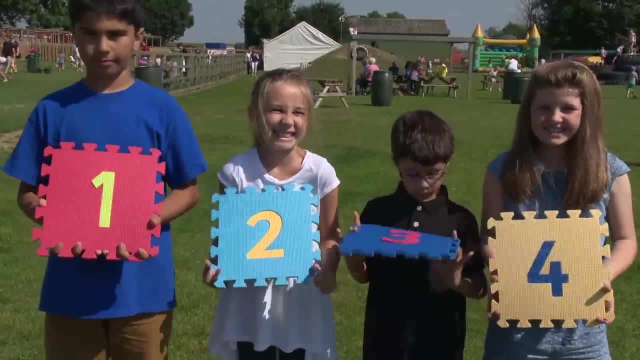 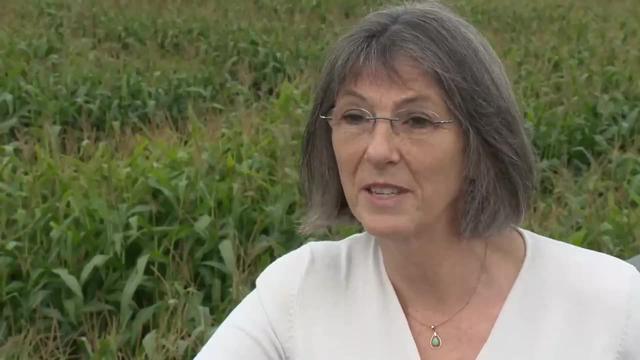 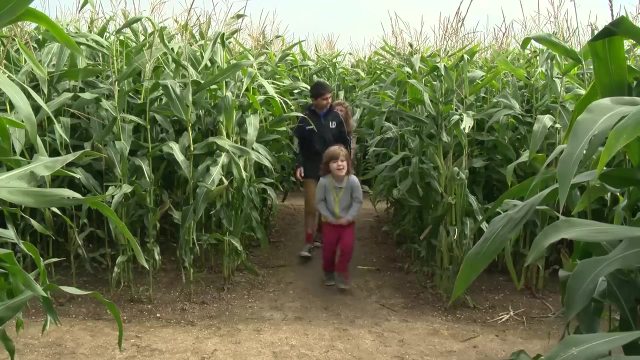 in context, stimulating to teach and rich in science Substance for learners. What we want for the next generation of children is for them to be inspired by mathematics. We need mathematicians for the future, and so we want a curriculum which offers them an opportunity to understand and to apply their mathematics, as well as feel that they're